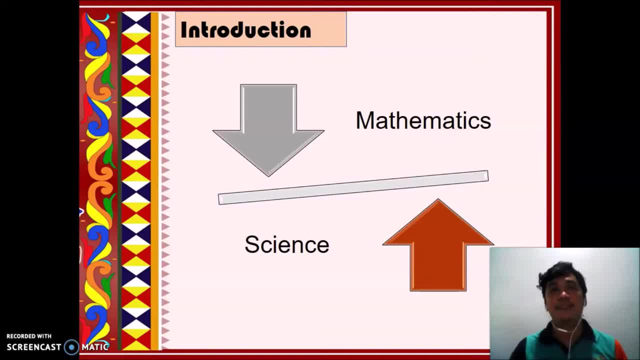 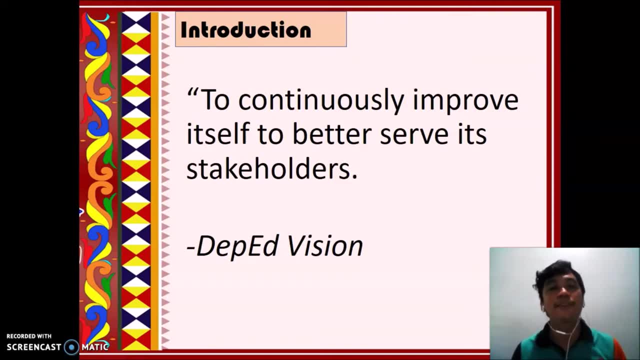 Are greatly associated with the concept of mathematics. A part of the vision of the Department of Education is to continuously improve itself to better serve its stakeholders, From the traditional way to more effective teaching strategies and approach, and every possible means were used by the institution just to improve the performance of the learner. 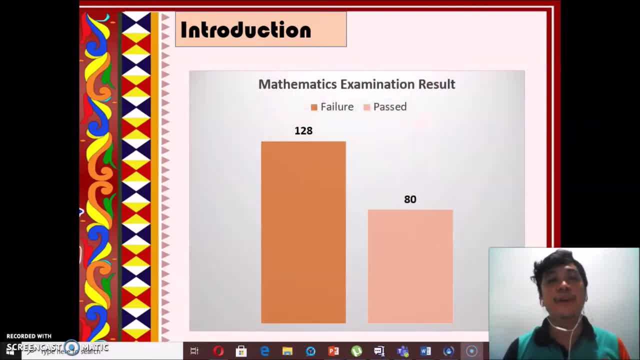 But despite the dream of the Filipinos to enhance the curriculum, the learners still failed to achieve competencies in the curriculum guide. In fact, in Tubud Central Elementary School, as per the error analysis done by the teachers per grading examination in mathematics, 128 in average failed the exam and 80 in average passed the examination. 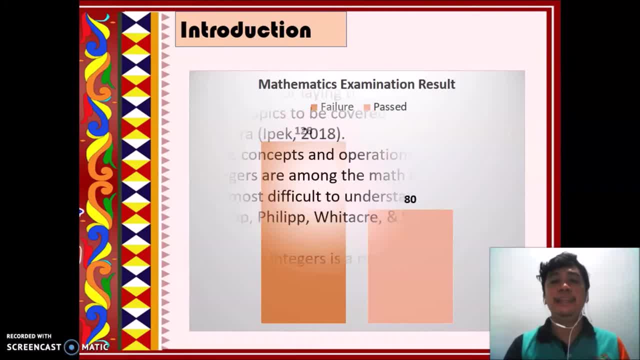 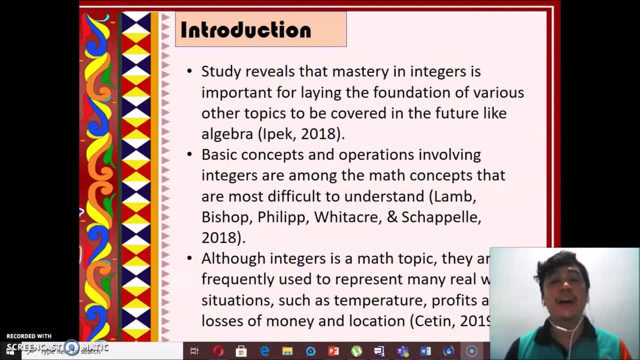 Now, one of the least mastered concepts or competencies by the learners is the concept of integers. However, study reveals that mastery in integers is important for laying the foundation of various other topics to be covered in the future, like algebra And also basic concepts and operations involving integers. 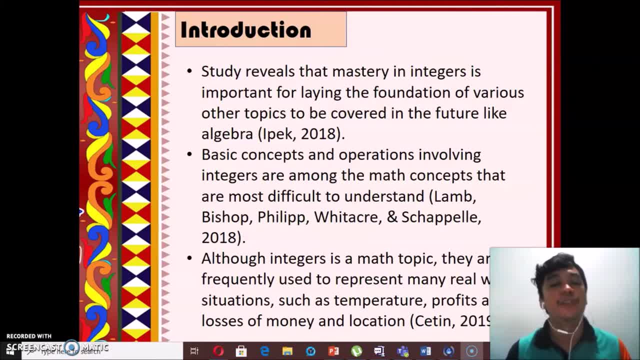 Are among the math concepts that are most difficult to understand, according to some studies. Although integers is a math topic, they are frequently used to represent many real-world situations, such as temperature, profits, losses of money and location. According to many studies, in mastering mathematical concepts like integers, both procedural skills and conceptual skills are very important. 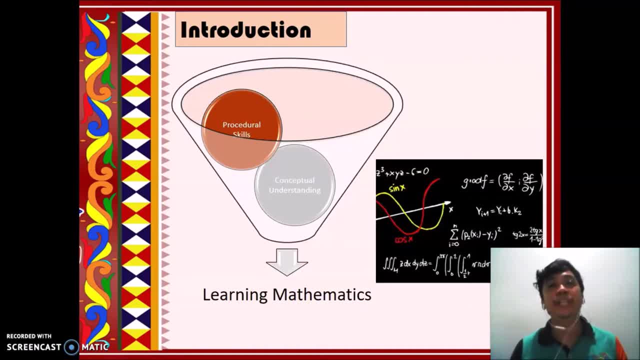 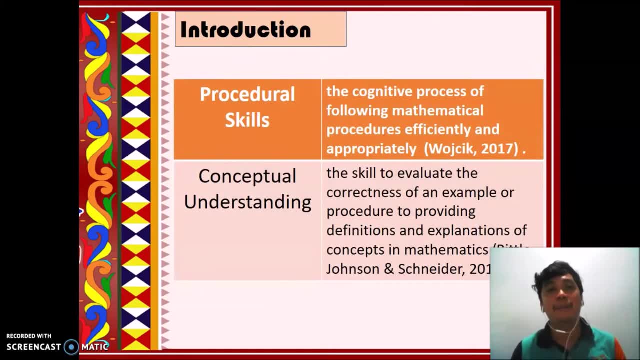 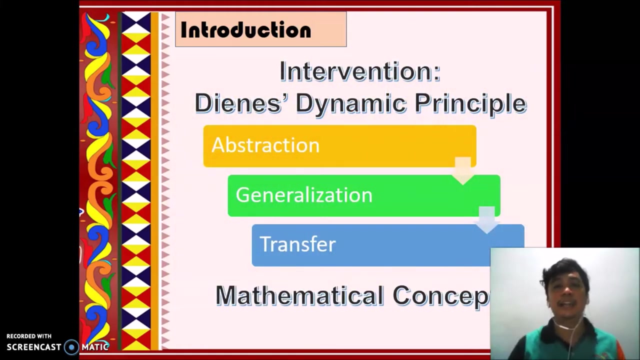 This is because procedural skill is the cognitive process of following the mathematical procedures efficiently and appropriately, While conceptual understanding is the skill to evaluate the correctness of an example or procedure, to providing definitions and explanations of concepts in mathematics. Now Cognizant to the conducted studies, it is imperative for teachers to employ strategies in their class that will both improve the conceptual understanding and procedural skills of the learners, with concrete materials that are faded into abstract representations. 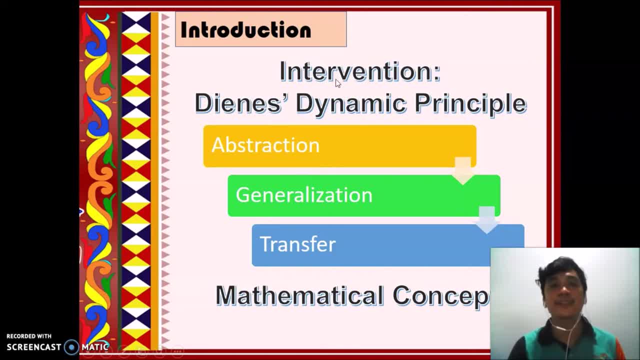 One of the best-proven strategies to employ this is to implement Zoltan Dienes' dynamic principle. This is because Dienes considers the learning of course to be the most important part of learning. He considers the learning of concept, of mathematics as a process which covers abstraction, generalization and transfer. 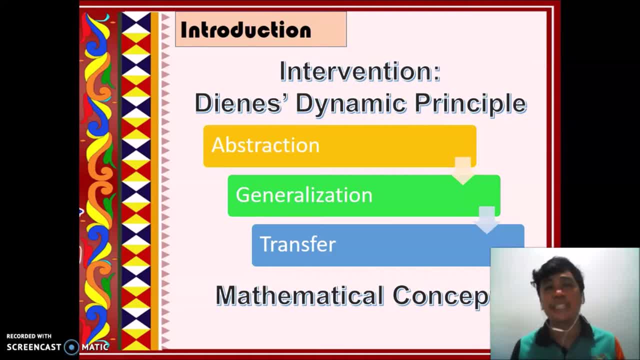 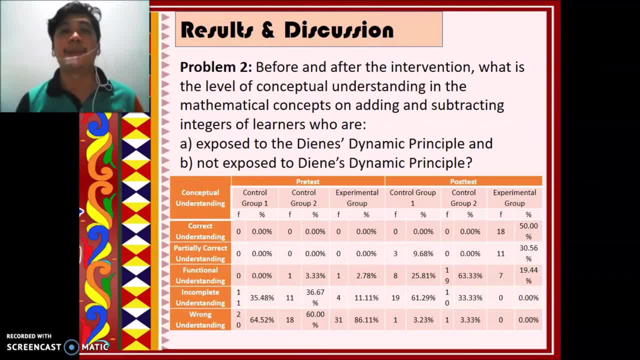 He developed a theory which focused on the use of discovery-type activities and learner-centered manipulative materials. mathematical concepts on adding and subtracting integers of learners who are exposed to diana's dynamic principle and not exposed to diana's dynamic principle, so the conceptual understanding. 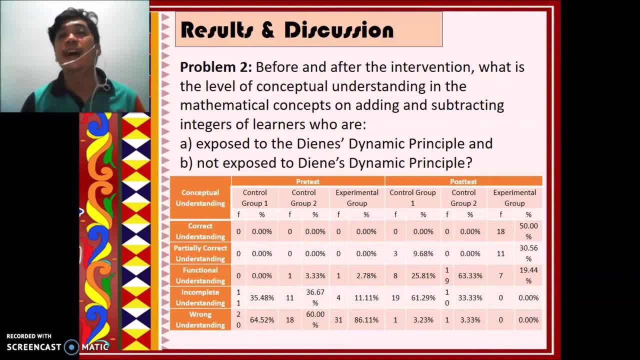 in adding and subtracting integers of the learners in the control and experimental groups in the icot is shown in this table. so according to the pre-test um scores of control group one, it revealed that 11 learners belonged to the incomplete understanding so and 20 learners belong to the 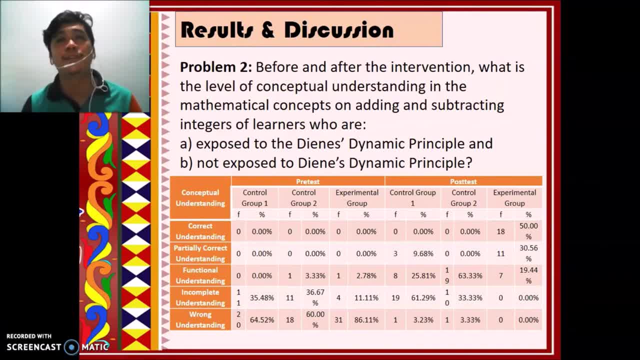 wrong understanding category, while in control group 2 one learner reached the functional understanding category and 11 learners the incomplete understanding category and 18 learners who belong to the wrong understanding category. moreover, in experimental group, one learner achieved the functional understanding category, four of them belong to incomplete. 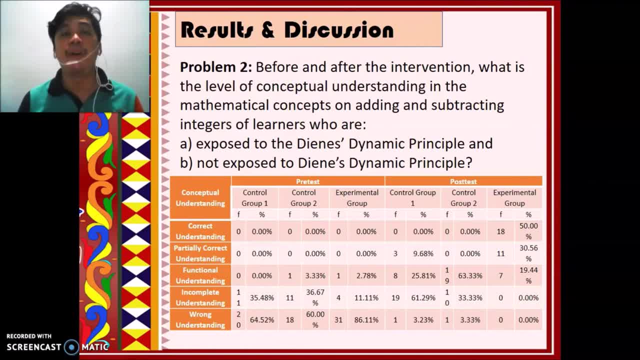 understanding category and 31 of them belong to the wrong understanding category in the pre-test. on the other hand, in the post-test results it showed that in control group one, three learners has reached the partially correct understanding category and in control group two has achieved functional cat understanding category 19 learners. here it is 19. 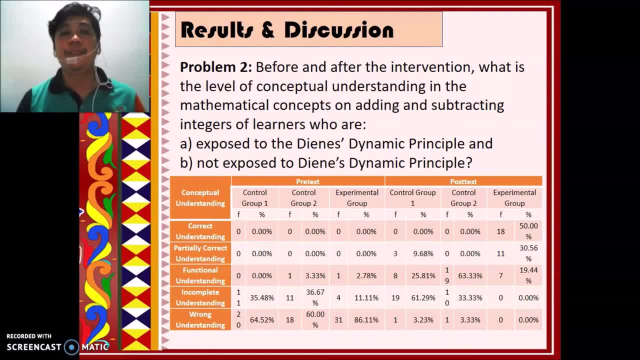 learners in control group two has achieved functional understanding category. However, learners in the experimental group has improved a lot in their conceptual understanding, wherein 18 and 11 of them have achieved the correct understanding and partially correct understanding category respectively. So that's it for the problem number two. 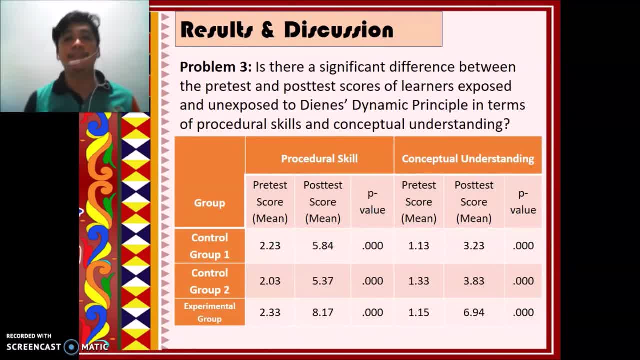 For problem number three, is there a significant difference between the pre-test and post-test course of learners exposed and unexposed to Deanna's dynamic principle in terms of procedural skills and conceptual understanding? So, according to the paired t-test as shown in this table, there is a significant difference as per the p-value, as we may see, 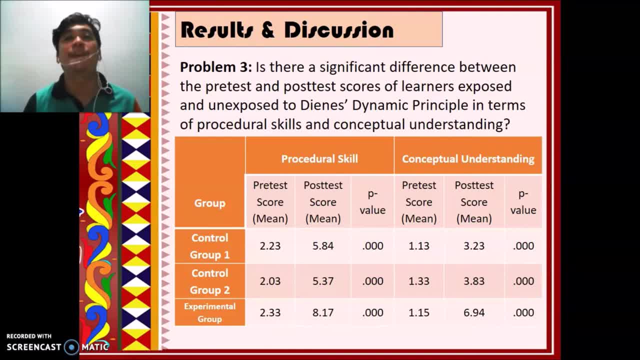 There is a significant difference between the pre-test and post-test course of the learners in the control groups and experimental groups in terms of procedural skills and conceptual understanding. However, it is noteworthy that the procedural skills and conceptual understanding of the experimental group is significantly better than the two control groups, as shown on their means of their post-test course. 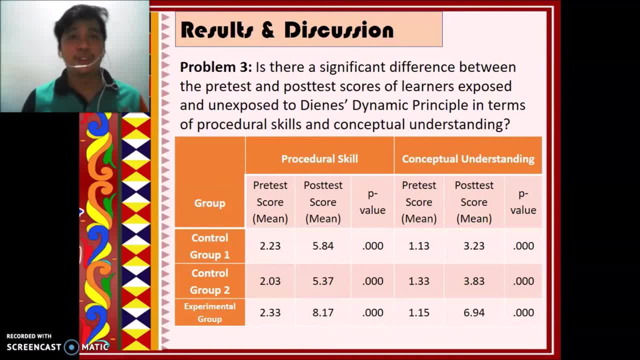 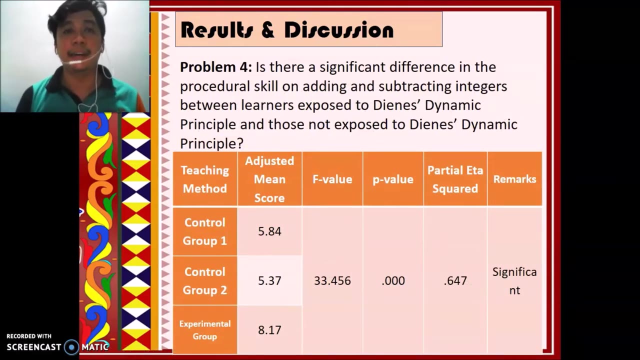 Hence the learners exposed to Deanna's dynamic principle have performed better than those who were not exposed to the strategy. So for problem number four. So is there a significant difference in the procedural skill on adding and subtracting integers between learners exposed to Deanna's dynamic principle? 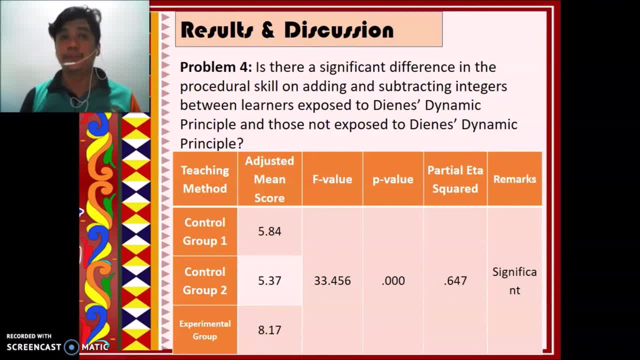 principles and those who are not exposed to dna's dynamic principle. so the analysis of covariance, or encova, reveals that there is a significant effect of the between subject factors factor groups we um through the p value or, as we can see here, point zero, zero, zero, which is less than 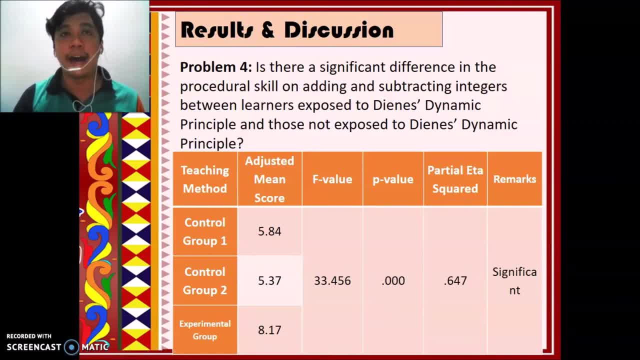 the cronbach alpha of 0.05 adjusted mean scores also suggest that the implementation of dna's dynamic principle is significantly better in enhancing learners procedural skills compared to the dna's dynamic principle, which is significantly better in enhancing learners compared to traditional method in group one and control group two. furthermore, um 65 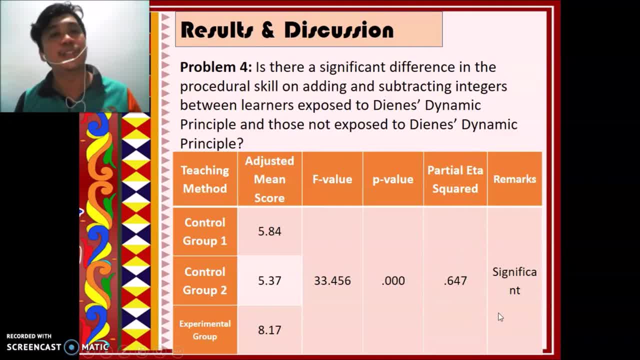 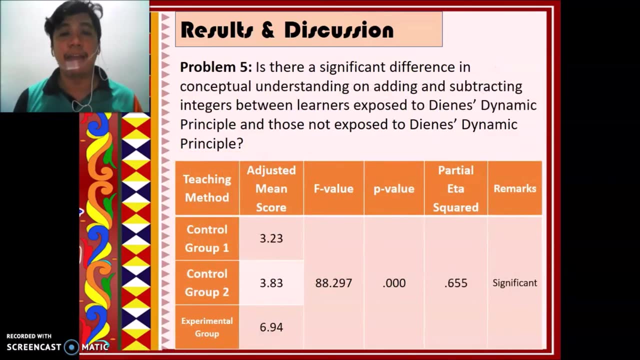 of this difference can be attributed to the intervention, which is dna's dynamic principle, as we can see in the partial error squared here, which is 0.647. problem number five: is there a signal of dual Whoo Service result of a those who are not exposed? 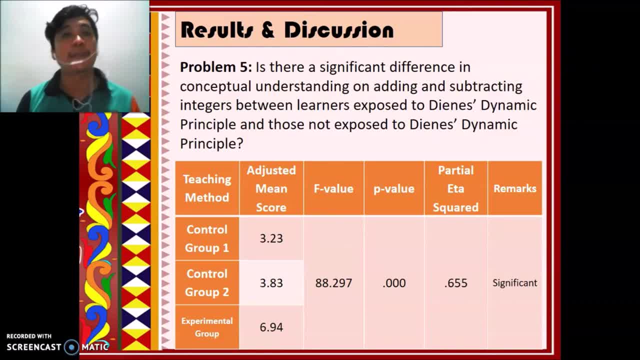 to dna's dynamic principle. again, the result of the test between subject effects in terms of conceptual understanding, as shown on this table, using analysis of covariance, revealed that there is a niceURL in which there is a subpor resisting be generated. that was been generated, directed at. 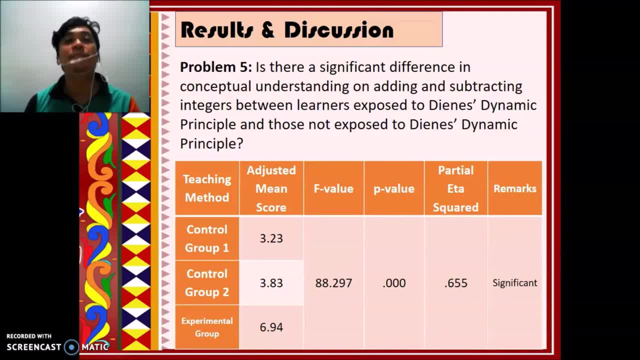 that there is a significant effect of the between subjects factor group because, as seen in the p value, which is 0.000, which is less than the Cronbach alpha of 0.05.. Adjusted mean scores also suggest that the implementation of Deanna's dynamic principle was significantly better in 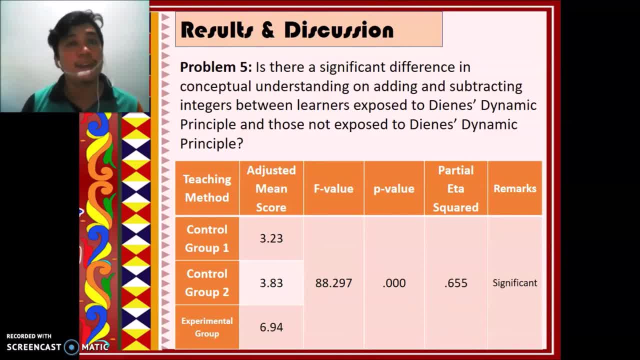 enhancing learners conceptual understanding compared to traditional method in control groups 1 and 2.. So we can see here in their adjusted mean score. Furthermore, 66 percent of this difference can be attributed to Deanna's dynamic principle, as we can see here in the partial eta squared which 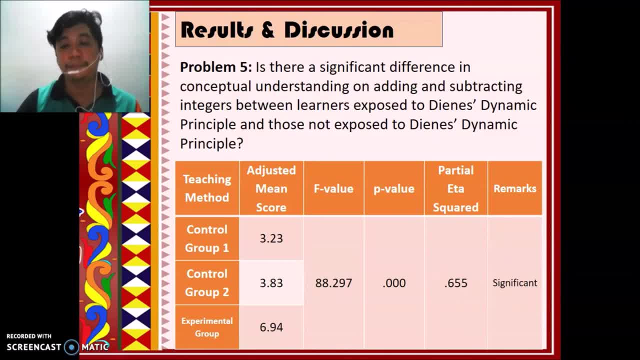 is 0.655.. Okay, so you can see that the difference between Deanna's dynamic principle and Deanna's dynamic principle- also results of this study- showed that Deanna's dynamic principle is an effective approach in improving learners procedural skills and conceptual understanding in adding and subtracting in teachers. 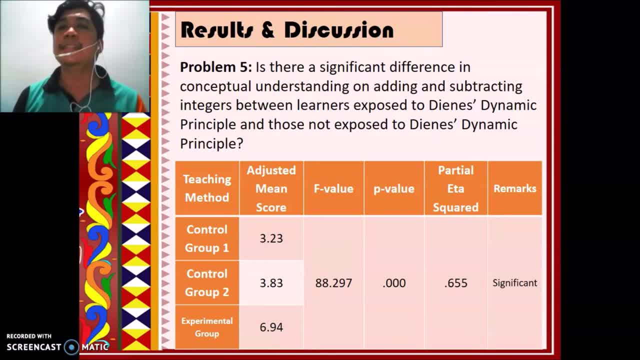 so this is because exposure to the in play, semi-structured and structured learning episodes of this teaching strategy allows learners to improve their procedural skills and conceptual learning. In addition, learning and trial and error are the fundamental factors that allow learners to concretize abstract mathematical concepts through the use of play and manipulatives. hence, 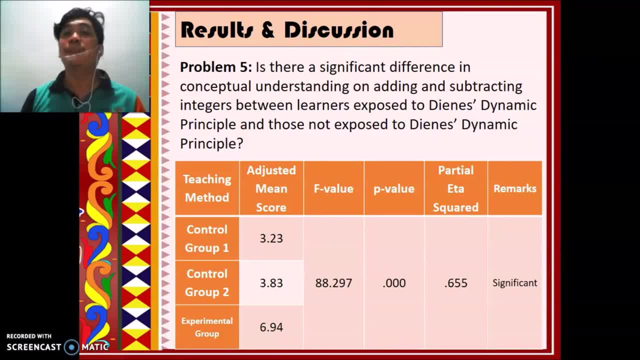 enhancing not only their procedural skills but also their conceptual understanding. So with this concretion, learners are able to solve mathematical equations and problems using different approaches. In fact, or in the recent research some of the students that were interested in mathematical equations, we have seen that there is a tendency to use any method-based method, such as semantics. So concretizing abstract mathematical concepts is surely not the only way to achieve its goals해주. 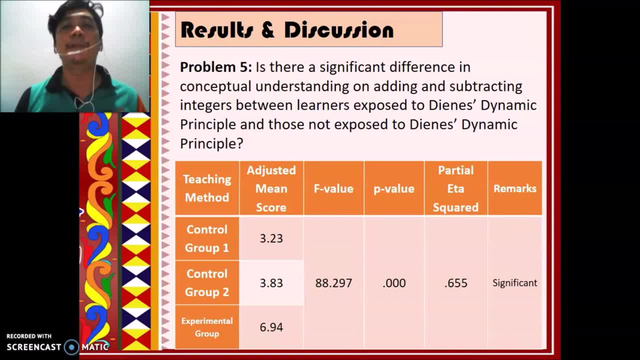 So concretizing abstract mathematical concepts and manipulatives. its ducking ability to use plays and manipulatives has been echoing through to the use of network modeling and AI skills: solve mathematical equations and problems using different approaches. in fact, uh, in the post-test. 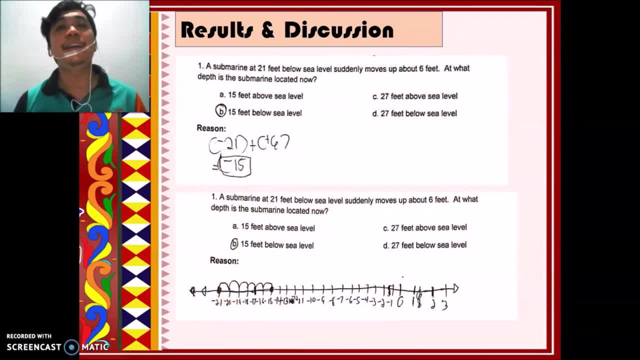 results of icot. it revealed that the learners provided variety of solutions for the mathematical problems they were tasked to solve. some learners, for example, in: in example number one in question number one. so this learner solved the mathematical problem using arithmetic. on the other hand, this learner solved the problem using model or the number line. in question number two, this learner 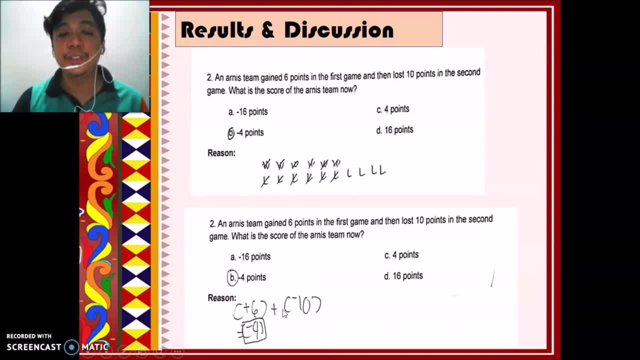 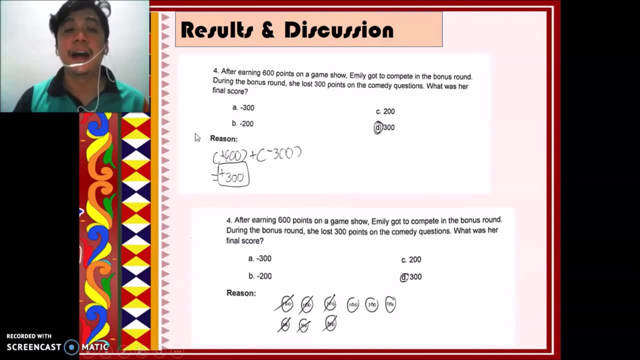 used drawing method and this learner used arithmetic method. and in problem four, this learner used arithmetic method and this learner used drawing or modeling method. so, um, in this sense, we can say that um the learner had developed, um their conceptual understanding in, because we can see that they have, they are, they have flexible solutions to. 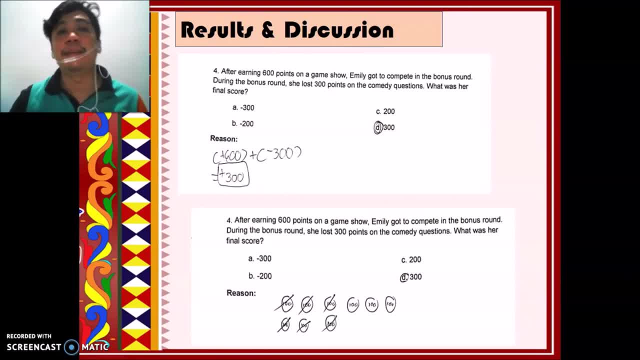 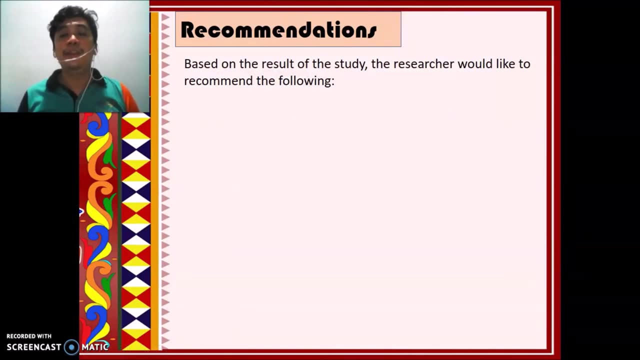 the same problem. so that is the the goal of mathematics: to improve the critical thinking skills and creative thinking skills of learners. okay for my recommendation. so, based on the result of the study, the researcher would like to recommend the following: number one: provide mathematics teachers training on the integration of dns dynamic principle on the. 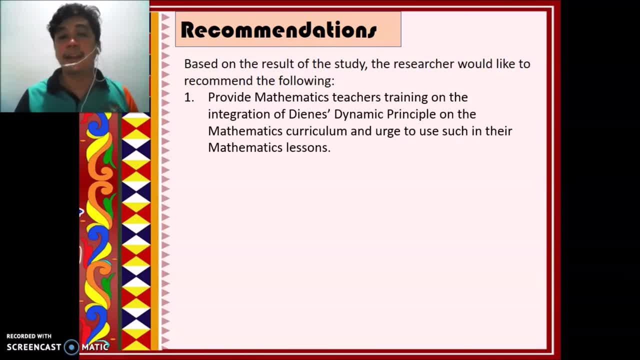 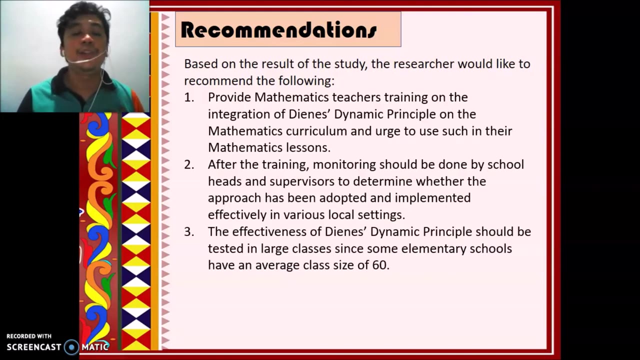 mathematics curriculum and urge to use such in their mathematics lessons. number two: after the training, monitoring should be done by school heads and supervisors to determine whether the approach adopted and implemented effectively in various local settings. number three: the effectiveness of dns dynamic principle should be tested in large classes, since